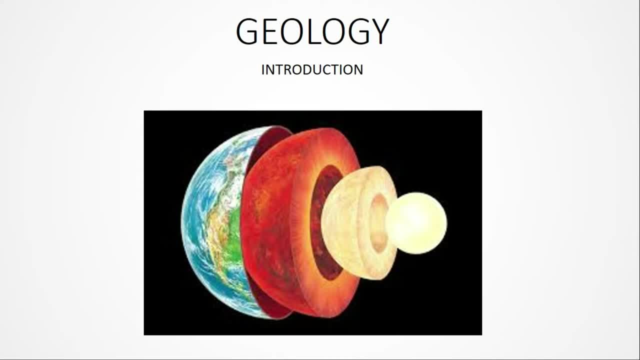 lecture on the internet which actually taught geology in an integrated and dedicated manner. See, at one place you may find someone teaching a separate topic of geology, someone teaching only a single branch of geology, but no one has actually taught the whole syllabus covering 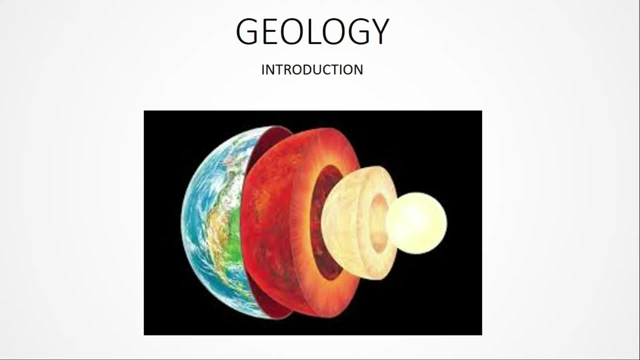 all the branches, all the topics of geology in an integrated manner, on a single window, on a single channel. So through these lectures, I am actually going to provide you all the basic concepts, All the topics, Topics covering all the major branches of geology- all together in a single channel. 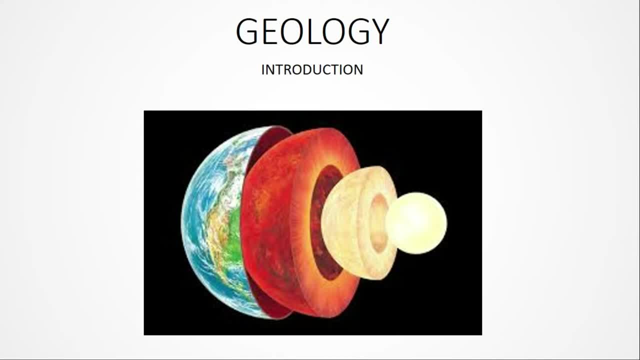 Okay Now, if you are doing your undergraduate bachelor of sciences from geology, or post graduation from geology, or even if you have taken geology as your optional subject for UPSC examinations, I think these lectures are going to help you really very well, because 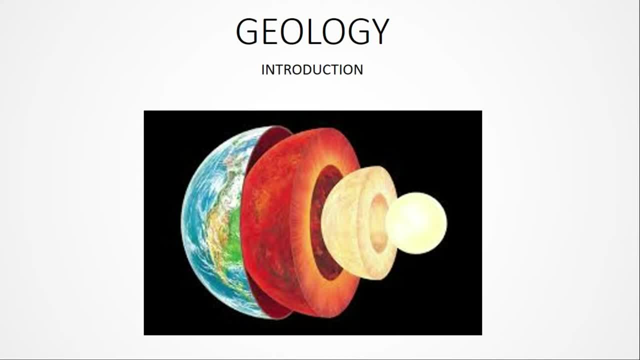 it is very knowledgeable to all the concepts and all the questions which could be asked from geology I am going to cover in all these lectures. So this is the first video where we are talking about the Introduction of geology. It is an 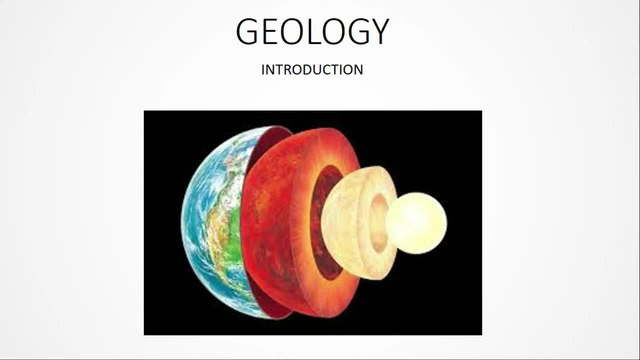 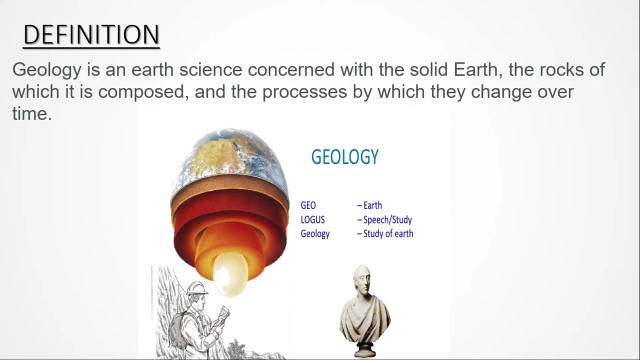 introductory lesson. Here we are going to study, we are going to see that, what are all the topics and branches which we are going to cover in our further lectures and what actually geology is. fine, so now let's start at first with the definition of geology. okay, so let's. 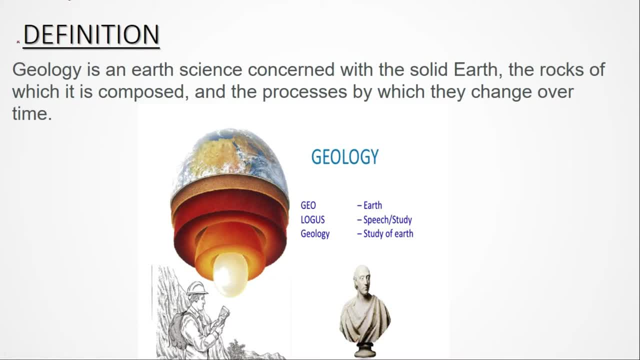 have a look at the definition. so geology is actually made up of two words: geo and locus. geo means earth and locus means speech or study. so, friends, geo plus locus is what you get as geology, and geology is that study of Earth. right now, let's 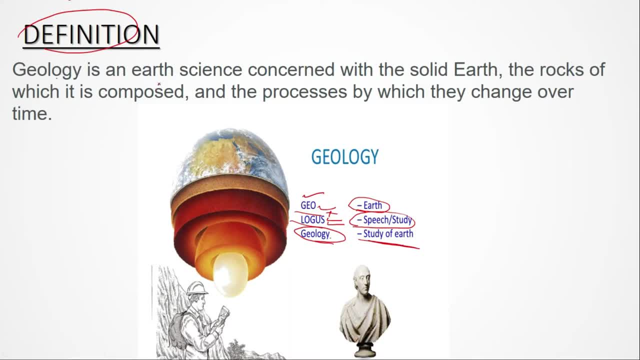 look at the definition: geology is an earth science concerned with the solid earth, the rocks or which it is composed and the processes by which they change over time. in very simple words, if we talk about geology, it is the science which is devoted to the study of the earth. okay, so study or earth, study of earth, it deals with all. 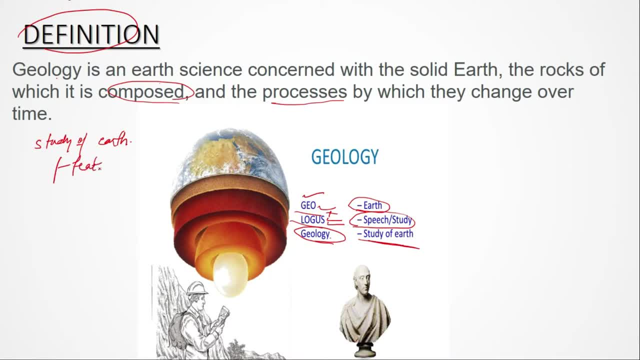 the features, features of the earth's surface. it is the study of the earth. it deals with the features of the surface: origin, composition, composition, structure and inhabitants of earth. fine, so geology is actually the study of earth, the earth's features related to the surface: origin, composition, structure and inhabitants of earth. so that is what geology. 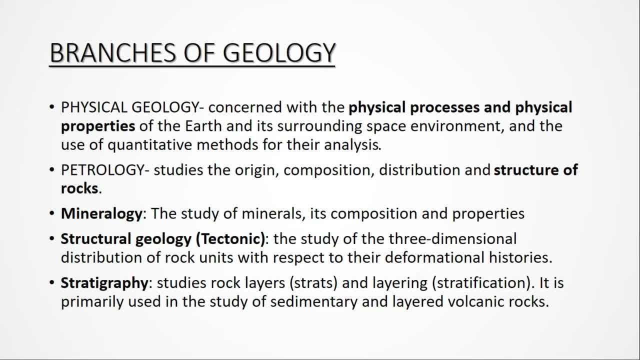 is now let's look at the important branches of geology. like like the other subjects, geology also has the branches of its own. fine, now, at first let's look at the first geology branch, that is, physical geology. physical geology is actually concerned with the physical processes, the physical processes and the physical 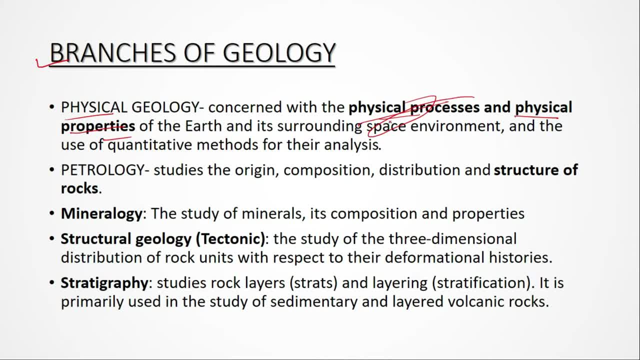 properties of earth, its surrounding space, environment and use of quantitative methods. quantitative methods for their left, using the physical and Hol乾ys coisas, and uses of quantitative methods for their left, using the specials from the planet earth andться winning the two analysis. so, in very simple terms, if we talk about physical geology, physical geology is concerned. 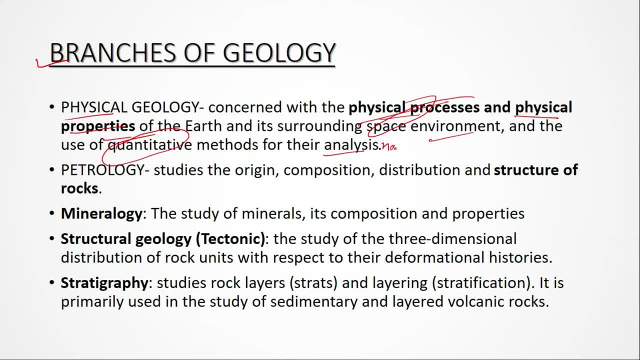 with the work of natural processes, natural processes which bring about changes upon the earth's surface. okay, after physical geology, let's talk about petrology. see in these in the first introductory lecture, where we are talking about the branches of geology. here we are not actually. 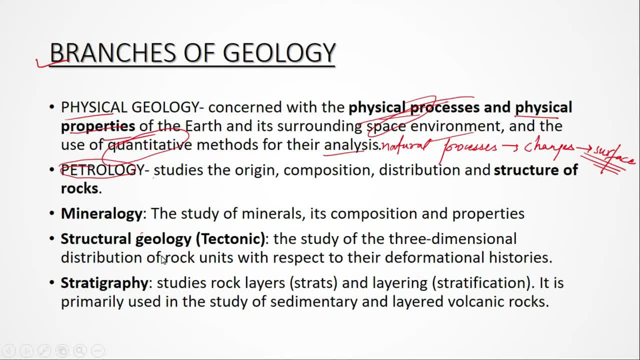 going very deep into them by, because here we are actually studying just a brief introduction of these branches. right afterwards, in the further learnings, we are going to talk about the branches. we'll be covering all these branches, the important topics and the syllabus under them separately. so just for now, no need to panic if you find any word which seems very difficult to you. 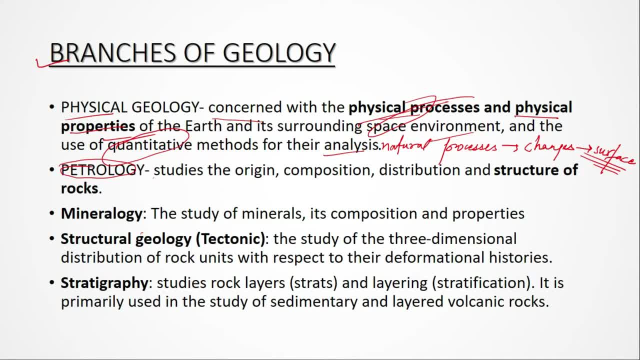 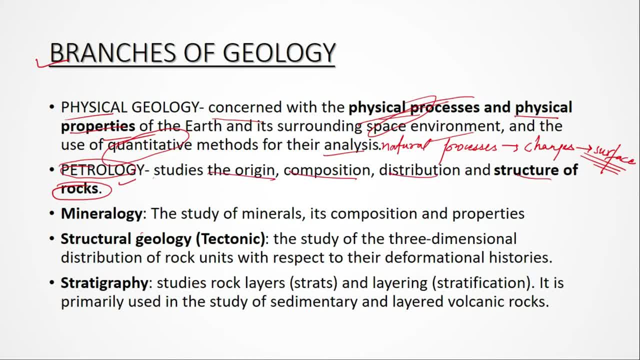 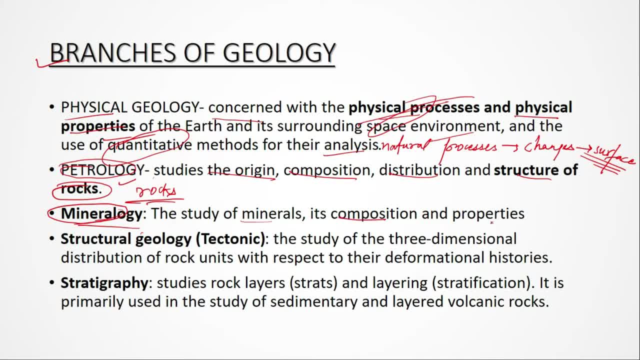 of minerals, its composition and properties. that is what we study in mineralogy: the composition and properties of minerals. fine. the next branch is structural geology. see the word structure here and structural geology. we are actually going to deal with the three-dimensional distribution of rock units with respect to their deformational histories or awaiting simple words. we can say: 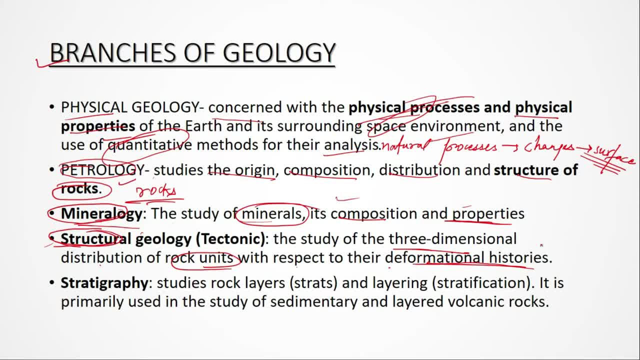 that it deals with the study of the structure of rocks. the name itself suggests that it is a structure of rocks. fine, see, our tectonic is used here. there's a topic: tectonic plates. in the further lectures there we'll be learning about what tectonic actually is for, and for now, just uh know. 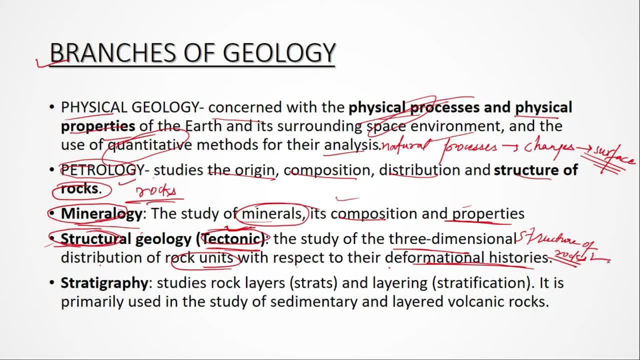 that that structural geology deals with the structure of rocks. and after that let's come to another branch, that is stratigraphy. see, stratigraphy is made up of the word strata. strata means layers. fine, so it studies the rock layers, stratas and layering. 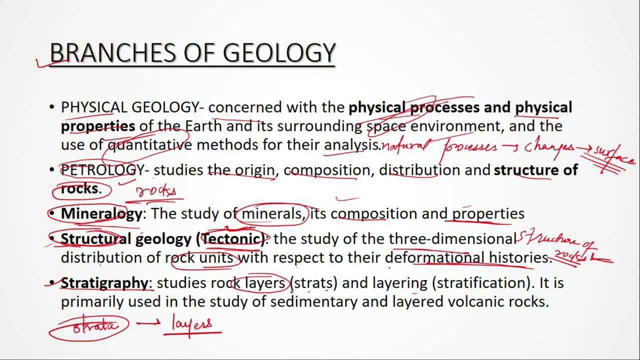 that is stratification. so the layers are are called as stratas and the layering is called as stratification. so it is primarily used in the study of sedimentary and layered volcanic rocks. see, when we will be studying about sedimentary rocks, they will study that sedimentary rocks are actually found in layers. 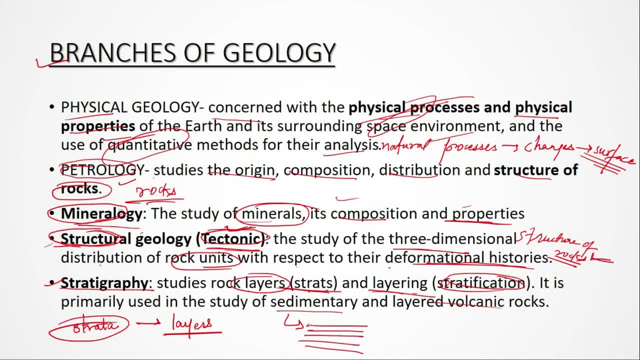 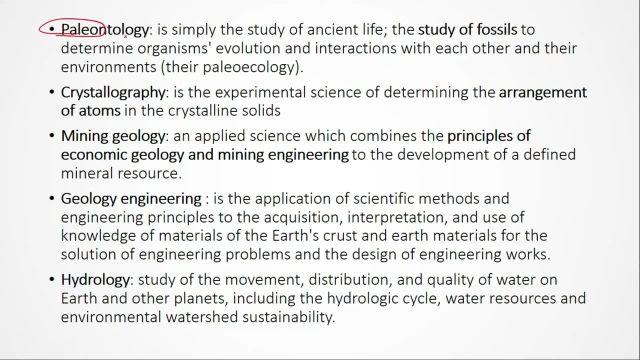 okay, that's why, in stratigraphy, we are actually going to deal with the sedimentary and layered volcanic rocks. so this is what stratigraphy is. the next important branch is paleontology- palaeontology- it simply deals with the study of fossils. okay, it deals with the study of fossils, so it is the same. it's simply the study of ancient 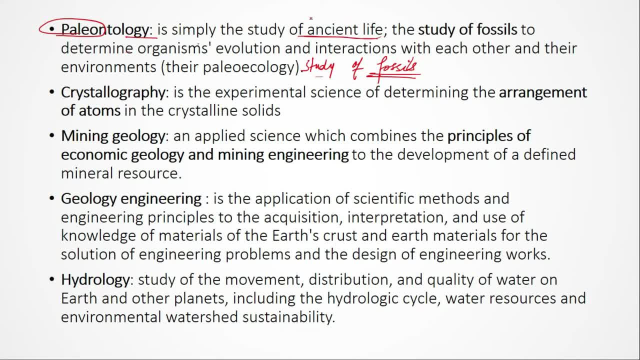 life. ancient life here doesn't mean those early man civilizations. fine. ancient life here actually means the fossils, the study of origin, and now we come to the study of meteorology. so so this is fossils to determine organism's evolution and interactions, the organism's evolution and 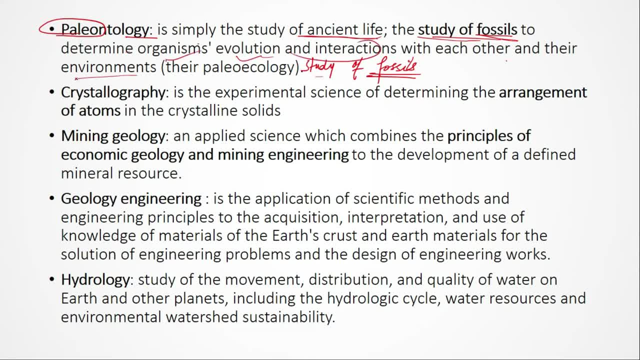 interaction with each other and their environments, which is also called as paleoecology, right. The next one is crystallography. Crystallography- something striking the mind related to crystals, right. So crystallography is the experimental science of determining the arrangement. 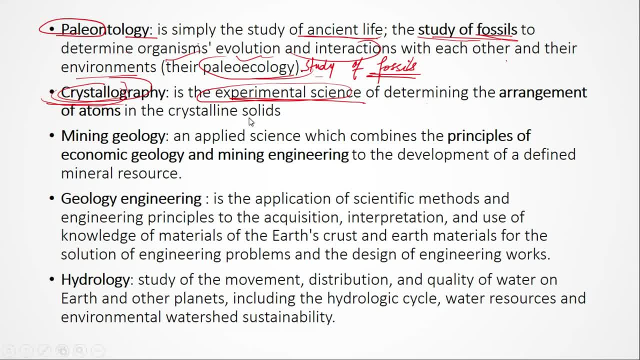 of atoms in the crystalline solids. So in crystallography we are actually learning about the arrangement of atoms in what? In crystals? Okay, Or say it: crystalline solids. Guys, don't look at my handwriting, I know it's not coming. 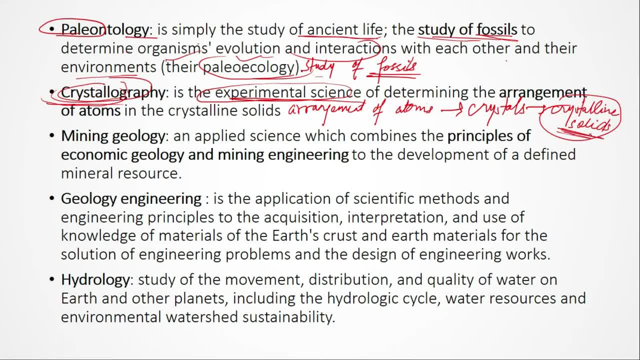 so neat, but I think you can understand it right. So, coming to another branch, that is mining geology. See guys, mining geology, engineering geology and hydrology. Okay, These are actually the applications of the other branches which we have already studied. 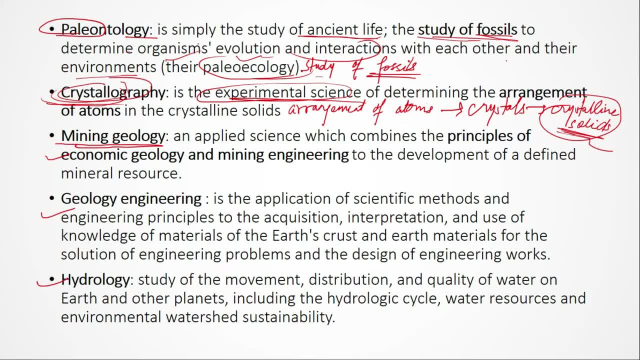 It is actually the application of geology which we are going to study in these branches. Okay, So first one is mining geology. It is an applied science. Just now I told you applications which what? which is related to what? The principles of economic geology and mining engineering. 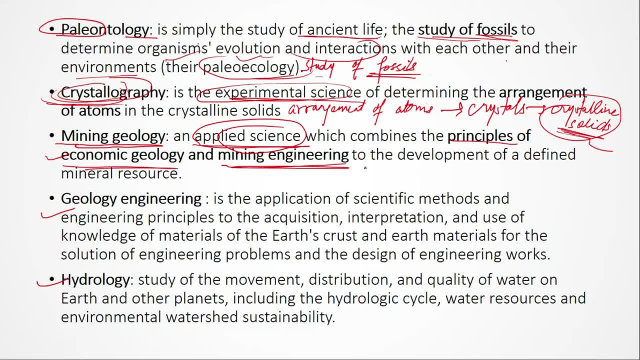 So, combining these two, Okay, Okay, So, combining these principles, we actually apply mining geology- Okay, To the development of a defined mineral resources. Regarding the minerals we will be actually covering, regarding everything about the minerals in the mineralogy and crystallography, And about 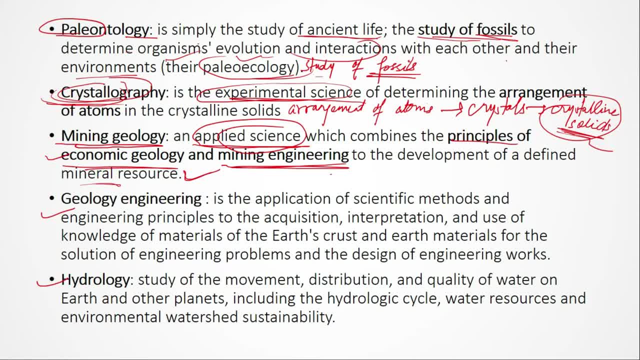 their further applications. we are going to study all these things in mining geology- Okay. The next is engineering geology. This is the application of engineering geology. Okay, It is the application of. it is also application based branch scientific methods and engineering. 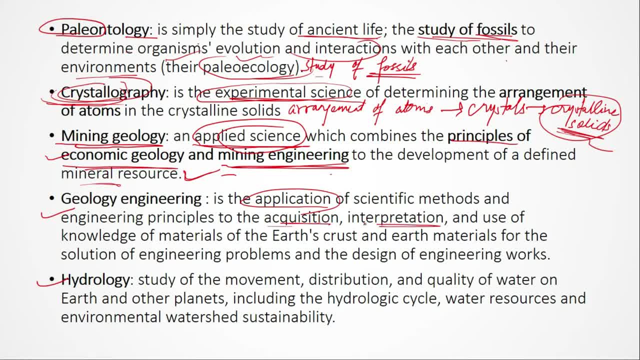 principles to the acquisition, interpretation and use of knowledge of materials of the earth's crust and earth's material for the solution of engineering problems and design of engineering work. It is actually related to engineering geology. So for the students who are actually doing graduation and post graduation here, you don't 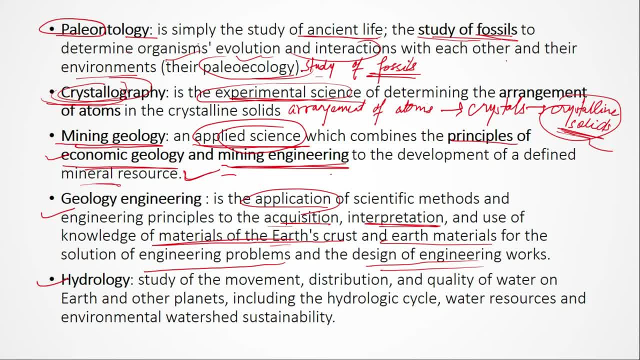 need to go much deeper about the engineering principles, but whatever it is related to the concepts of geology. we will be dealing all those things here, Okay, The next one is hydrology, Hydro. what? what is hydro? Remember something? Yeah, It is. 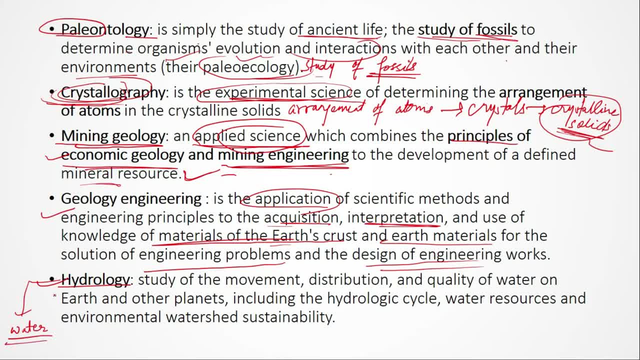 water. Hydro means water, So here we are going to study actually about water, Not not proper water, but, yeah, The movement, distribution and quality of water on earth and other plants. This is what we are going to study in hydrology, including the hydrological. 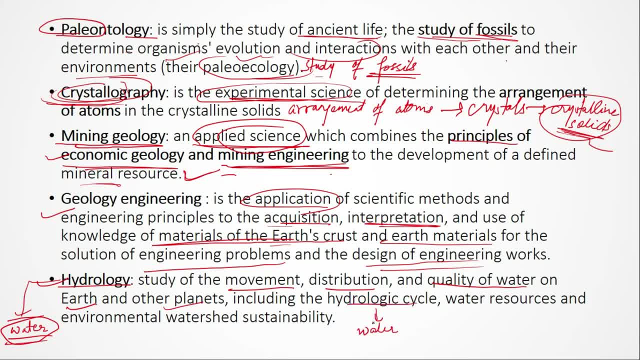 cycle. That is what The water cycle, water resources and environmental watershed sustainability- Okay. Sustainability, What Sustainable development, Realizing the resources without actually harming the environment? Okay. The needs of the future: Okay, That is sustainability. Now, if you are a geology student, it is really. 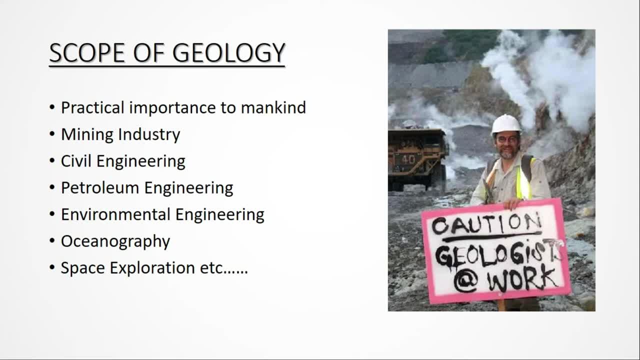 important for you to actually know what are the scopes of geology. All right, If you are planning to become a geologist or whatever, you should actually know that, whatever you are studying, what are its scopes, What are its practical applications and how it is important. 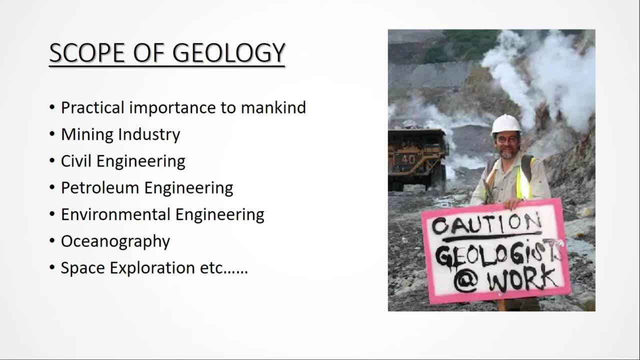 to the humans, to the mankind. Okay, So when we talk about the scopes of geology, the first thing we are going to look at here is that, see, it is of immense practical importance to mankind. How See in the previous. 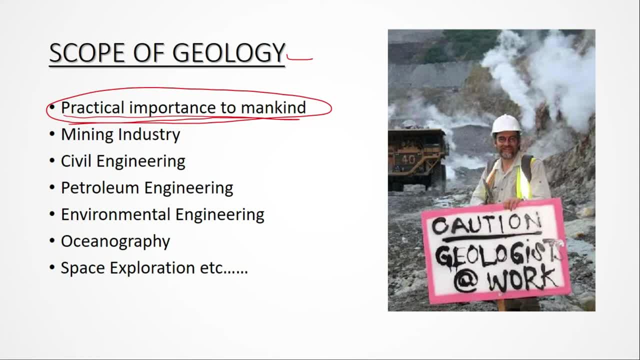 branches when I told you I had talked to you about the branches of geology. there we have seen many applications of some branches, like the mining geology, engineering geology and so on. So saying that geology is of practical importance to mankind means that it plays. 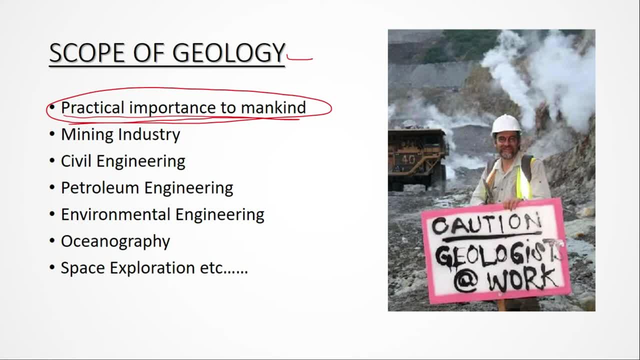 a very useful part in the search of important resources for the existence of mankind. See, it plays a very important role in search of coal, petroleum, minerals, atomic fuels, fossil fuels, right, And it is directly concerned with the ore, minerals, the industrial. 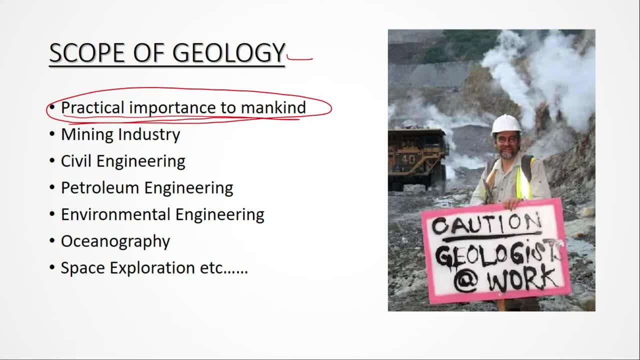 minerals, the mining industry. So if you talk about the economics, if you talk about the existence of mankind, so many things are related to geology. Fine, Like see, just here, in this mining industry, we have learned about the mineralogy, mineralogy we have. 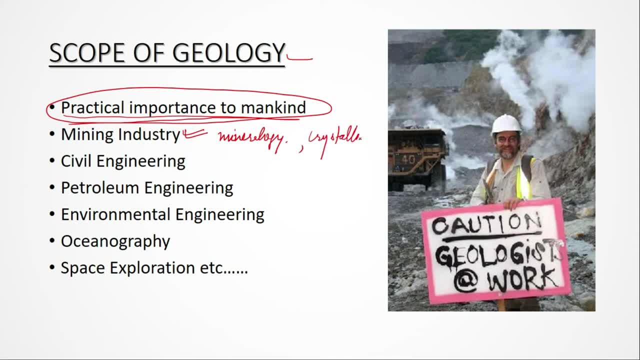 learned crystallography. I mean, we will be learning crystallography, mining and economic geology. So the principles of all these branches are applicable in the mining industry. The same goes with civil engineering: all the dams, bridges, tunnels. So what do you think? 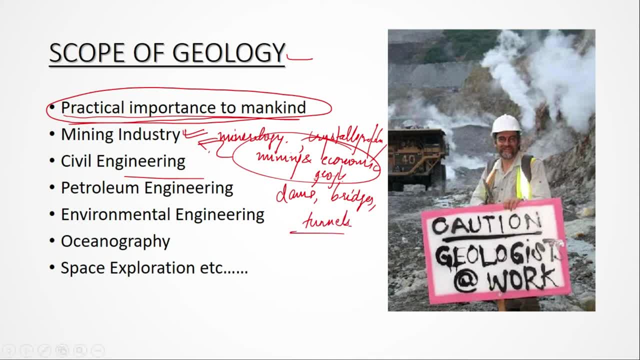 What these engineering do? Do you think they are applicable in the mining industry? Do they go anywhere around the world and at any region, they start digging up tunnels, they start making bridges or they start making dams. No, Actually, these all things when? 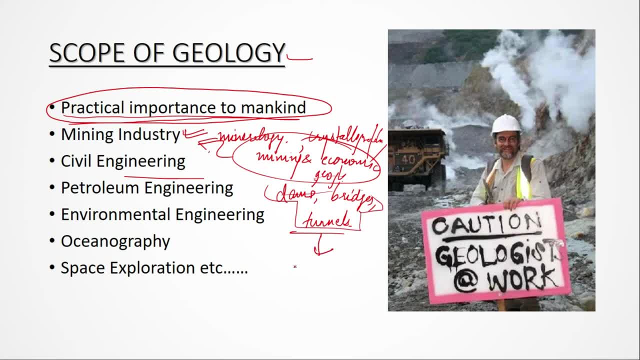 they are going to be constructed. at first we have to look at the geology of that region, right? So these important applications of geology are applicable in the mining industry, And these important applications of geology are applicable in civil engineering also. 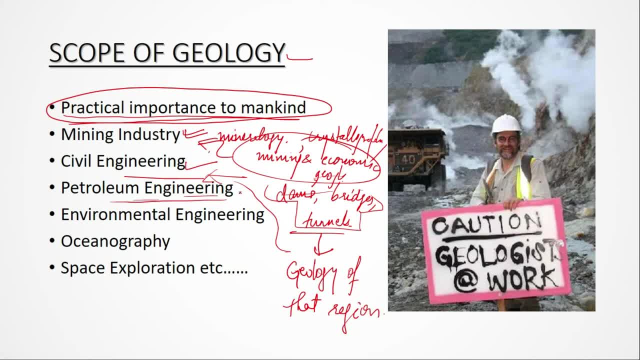 in petroleum engineering, identifying the areas where petroleum, where fossils can be found, where oil and natural gas can be found, where petrol can be found There. we are actually applying the principles of geology right In an environment: engineering in oceanography. 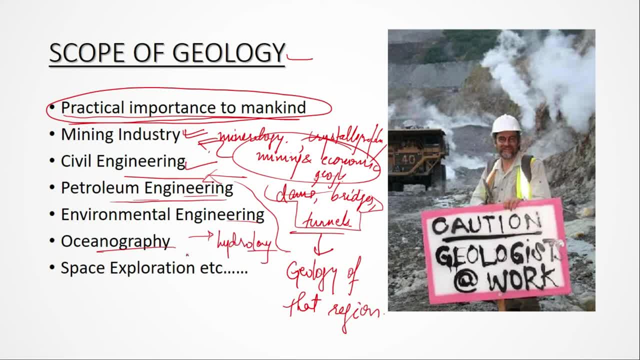 hydrology would be studied. Other things also. in oceanography you study about the marine life. also There you will get to know about some fossils, also In space exploration, something related to your physical geology. So I mean not a single branch of geology is applicable. 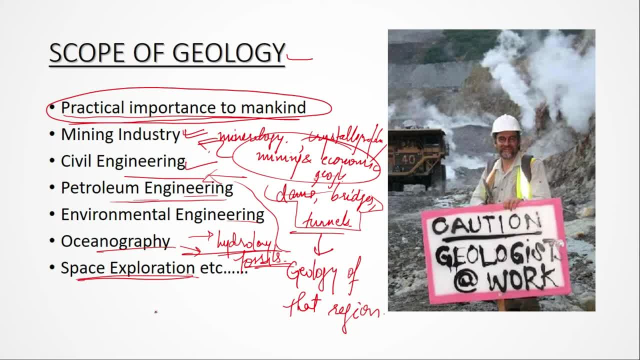 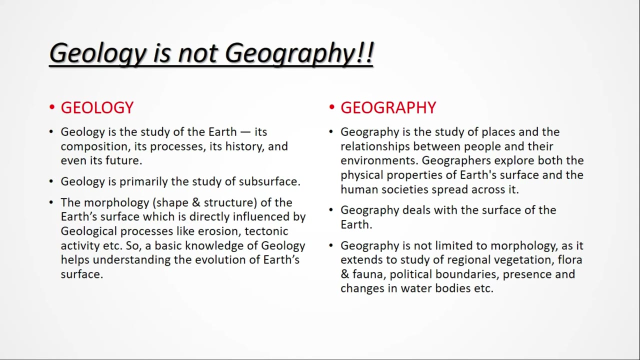 to each of them, but a combined knowledge of geology. combined knowledge of geology is necessary for all these scopes, right? So after the scope of geology, let's look at another very important, frequently asked question from the students that geology and 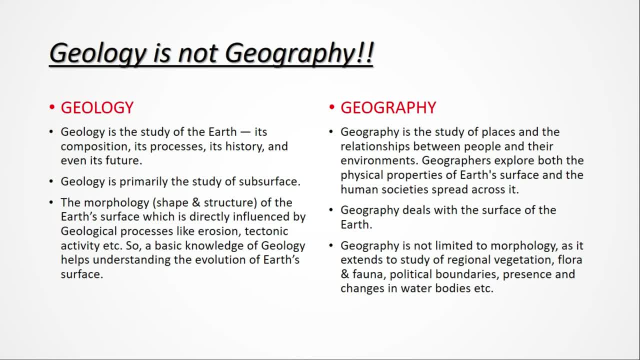 geography are same. I mean, whatever you study in geology, it's more or less same like geography. But, friends, no, geology is not geography. If you are a geology student or if you are a geography student, you really need to know the difference between the two. So let's. 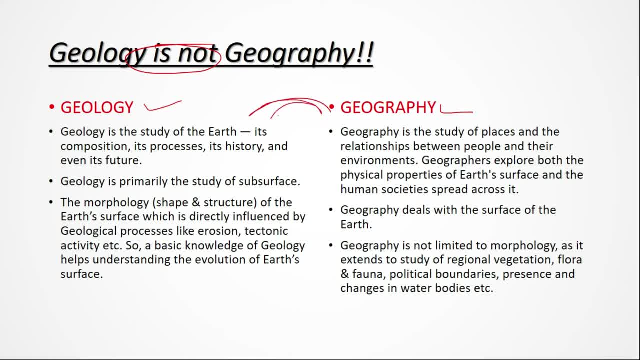 look at the first question: Why geology is different? Because they are not the same. Yeah, they have some similarities. They have some common topics in them, like the geomorphology- Geomorphology- that is the same topic in both geology and geography, But there are many. 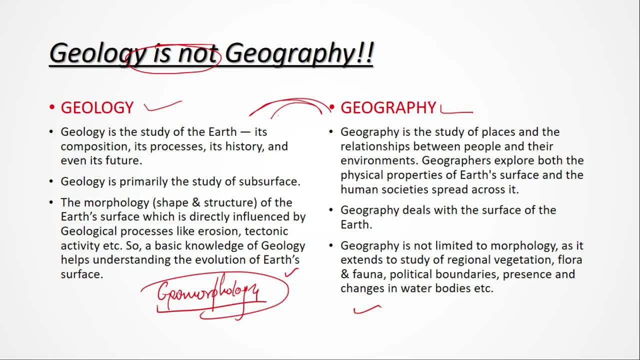 differences between them, and that's why you say that geology is not geography, right? Talking about the first difference, it's the definition: Geology is the study of the earth, its composition processes, history and even its future, right? so you are just here, mainly. 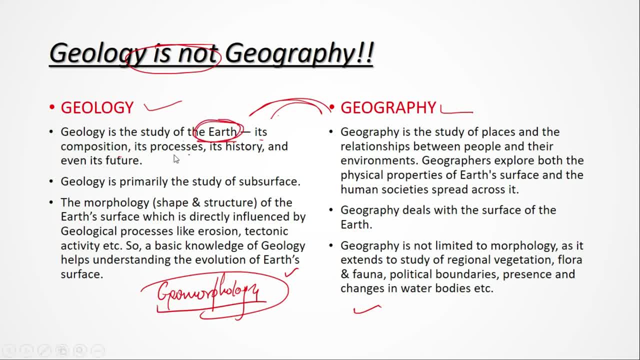 concerned about the earth composition, the processes going on. and so there you are. you are not concerned about the human and their relationship with the environment and all but in geography. geography is the study of places and the relationships between people and their environment. so basically, here you are, establishing a relationship between the 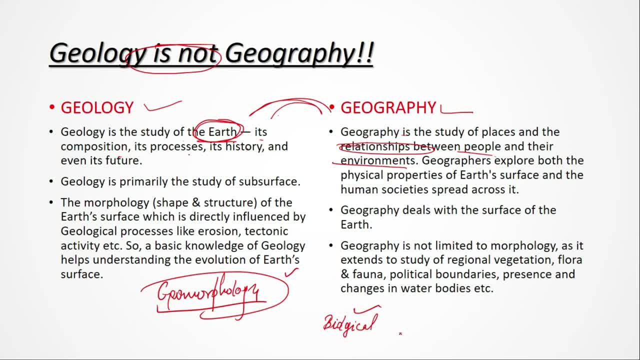 biological aspects as well as your environment. okay, so geographers explore both the physical properties of earth's surface and the human societies spread across it, you fine? so here you are actually concerned with the human societies, the flora, fauna, vegetation and all, but in geology that's not the case, okay. so next difference if you talk about is that 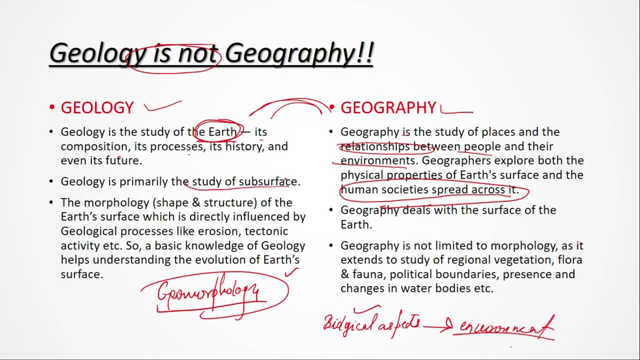 geology is primarily the study of subsurface, whereas geography it deals with the surface of the earth. here, the surface surface of the earth and geography, uh sorry. geology, the subsurface of earth and geography, the surface of the earth. fine now, in geology, the next important difference is that the morphology. morphology means the shape. 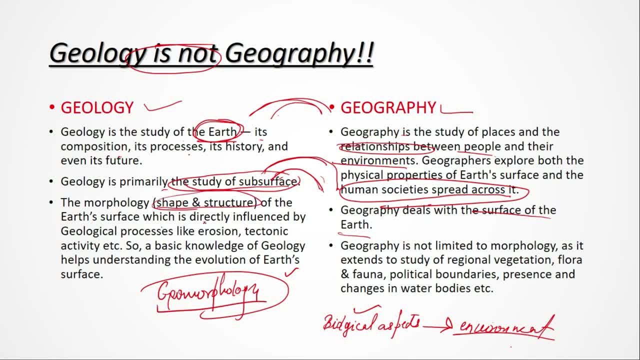 and structure of the earth surface, which is directly influenced by geological processes like erosion, tectonic activity, etc. these will be learning in the further lectures, don't worry so. a basic knowledge of geology helps understanding the evolution of earth surface. to understand the evolution of earth surface, you need to have a basic knowledge of geology, because 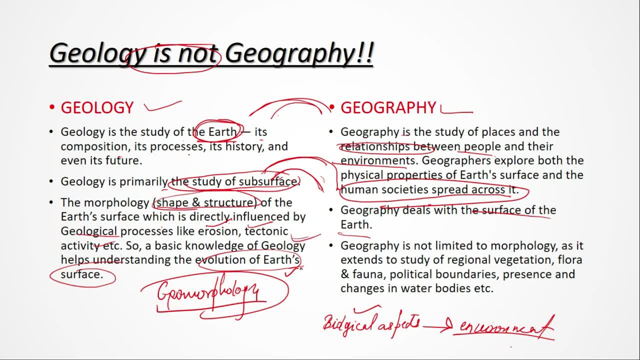 the evolution, erosion, origin, composition and all these all are linked to the uh: geology, not geography. i mean geography. you would be learning about morphology, see geography, but it is not limited to morphology as it extends to study of regional vegetation, flora, fauna, political boundaries, presence and changes in water bodies, etc. in geology, you are not going to learn about the vegetation.